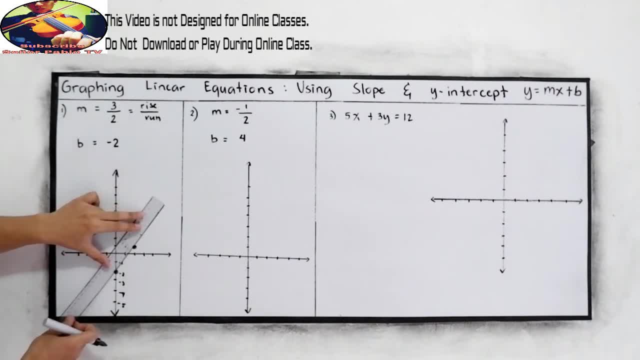 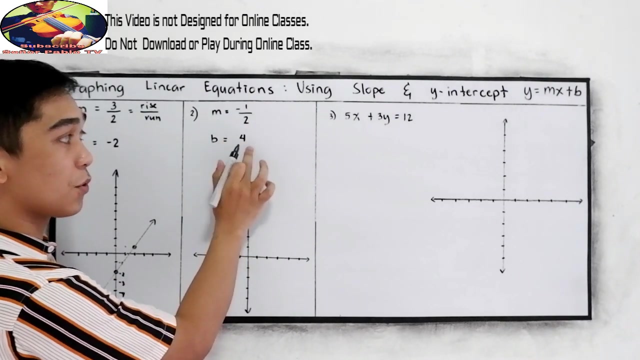 This will be our two points. We are now ready to connect the points. This will be our graph. This will be our graph. Let's try number two: m, or the slope is equal to negative 1 half, and b, the y-intercept is equal to 4.. 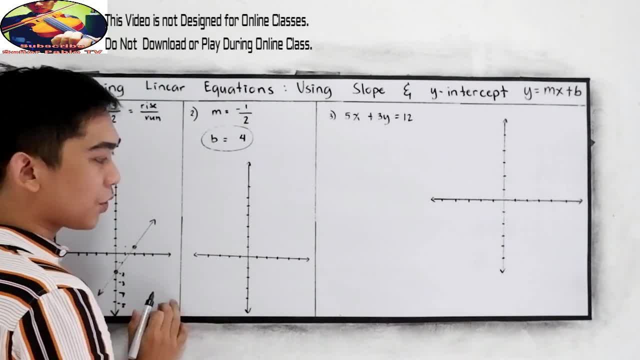 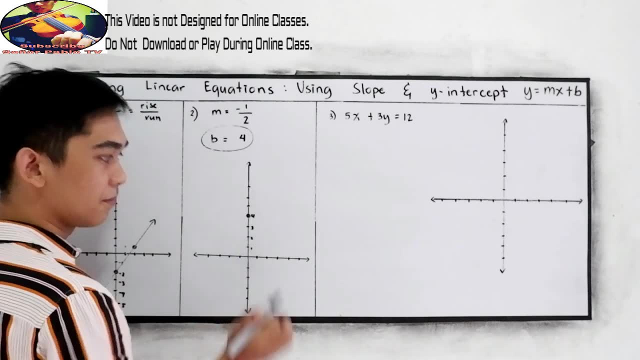 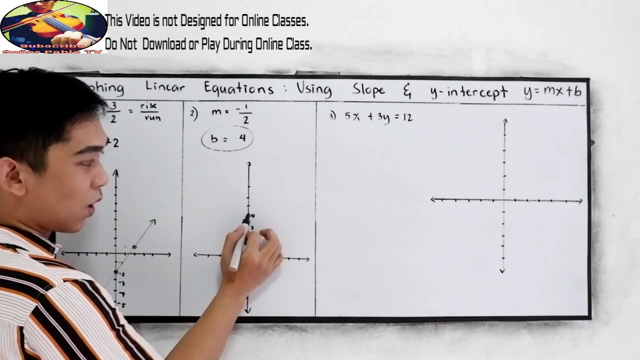 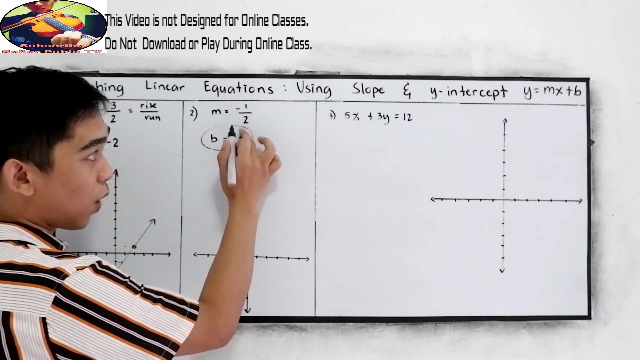 Locate our y-intercept positive 4,, so positive 1,, 2,, 3, 4.. That would be our first point Now. 1 over 2.. So 1 over 2.. So 1, rise negative. so we will go and run to the left twice. 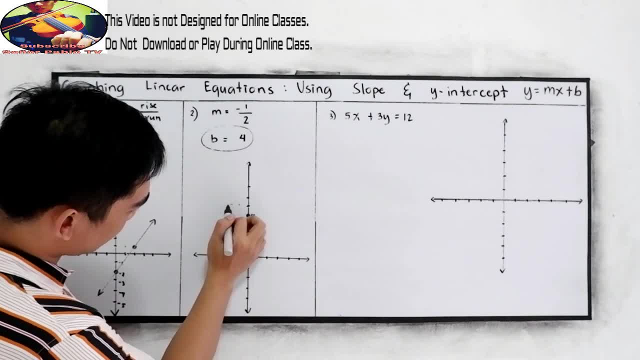 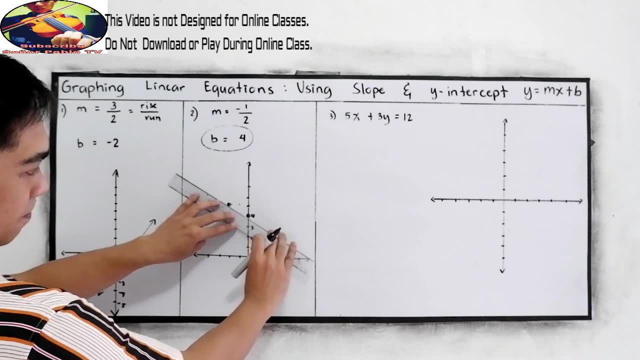 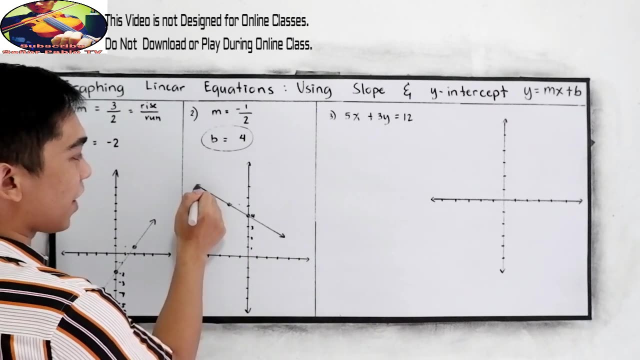 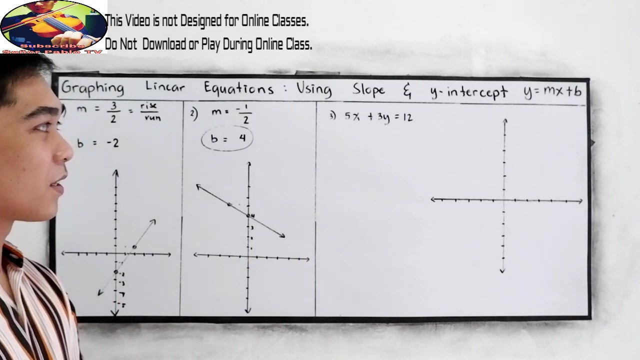 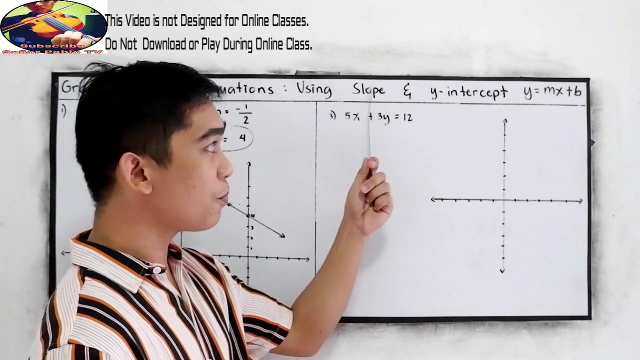 So 1, 2.. Points is located, 2,. okay, Now connect the points. This will be our graph. And for our third example, 5x plus 3y is equal to 12.. In this case, let us find our slope and our y-intercept. 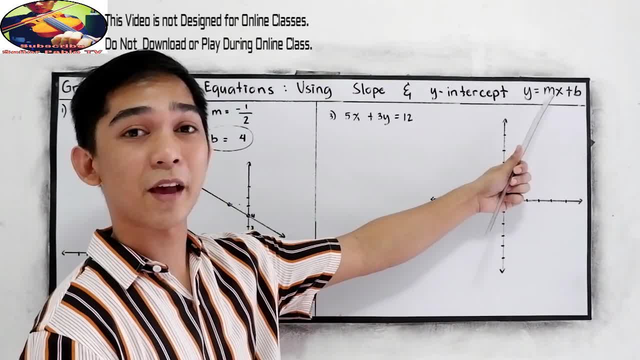 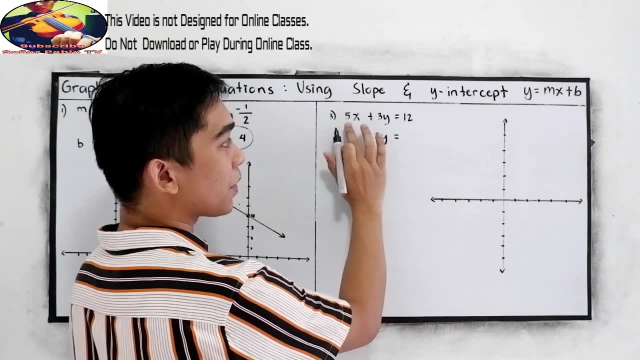 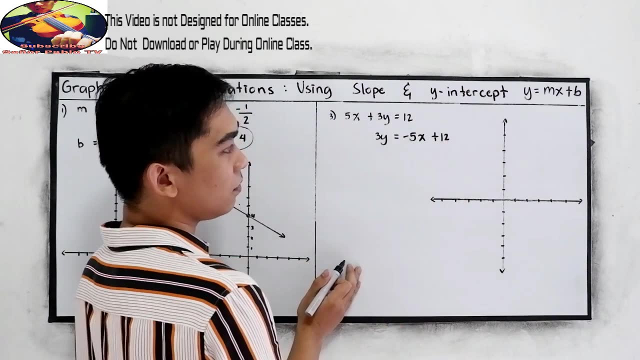 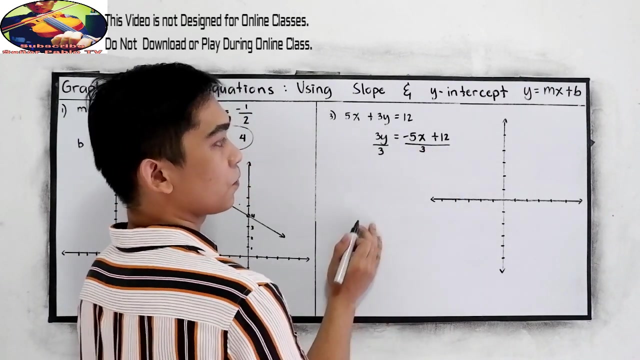 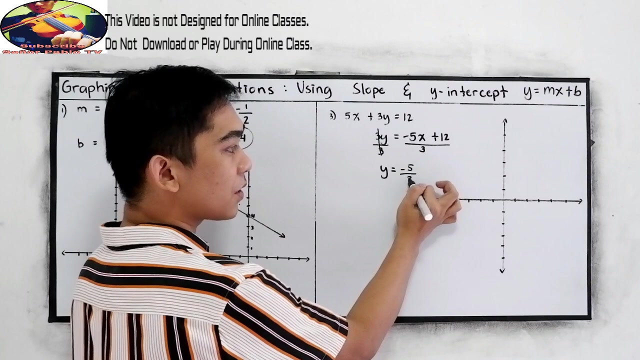 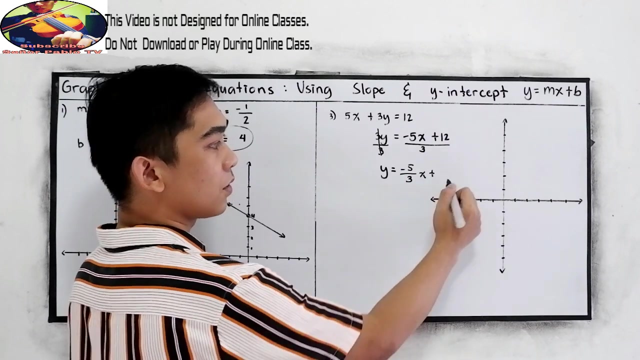 Let us first write into slope-intercept form. So 3y is equal to addition. property of equality Negative 5x plus 12.. Now to find y, divide the equation by 3.. And so y is equal to negative 5 over 3x plus 12 divided by 3,, 3,, 6,, 9,, 12.. 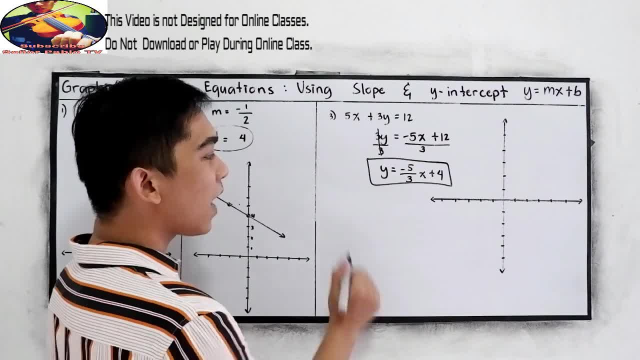 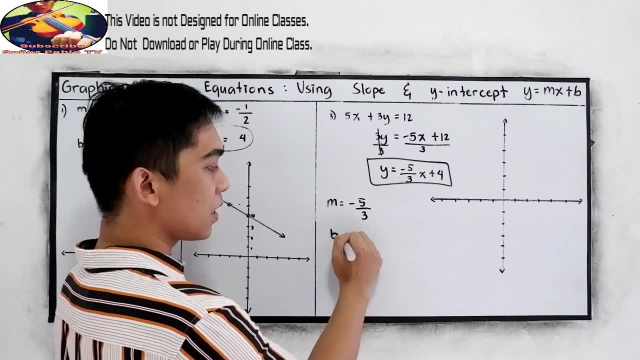